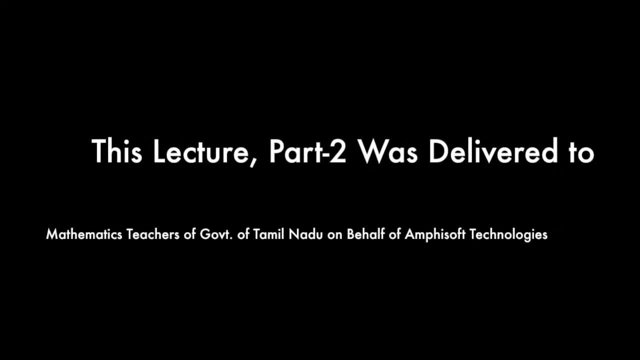 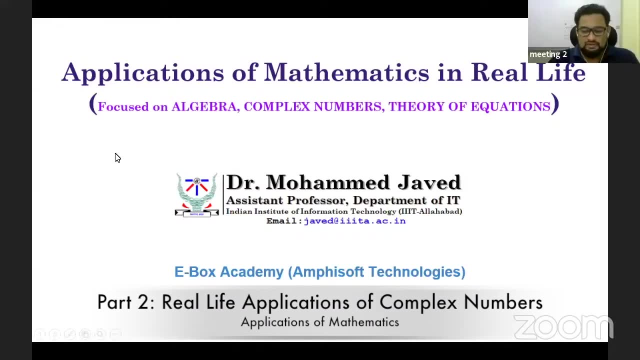 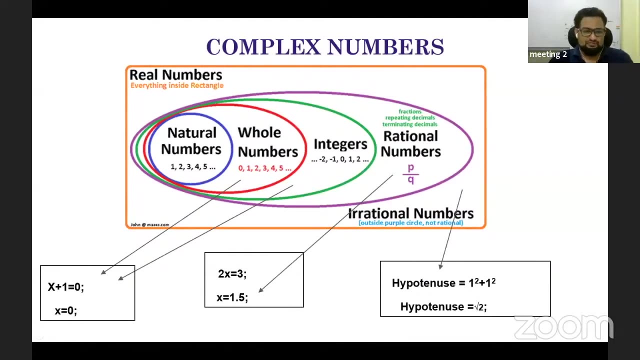 This is a very important area of mathematics. So let us try to understand this complex number from two perspectives. First is the mathematical perspective and second one is the philosophical perspective. So we have natural number. Let us assume that we have natural numbers, The 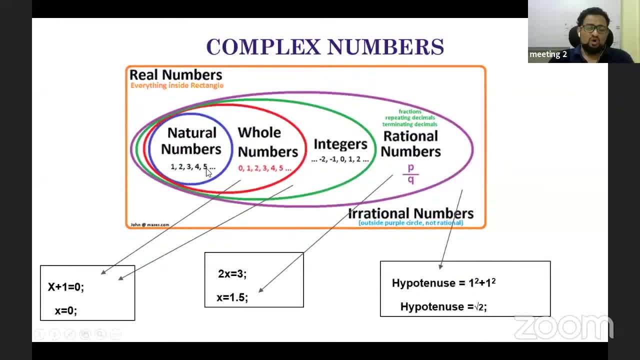 natural numbers: 1,, 2, 5.. Now, when we are solving any equation, any mathematical equation, we feel that there are also some equations of this type called x plus 1 equal to 0 or x equal to 0. So this necessitates that it is not that only natural number will be enough for me to solve. 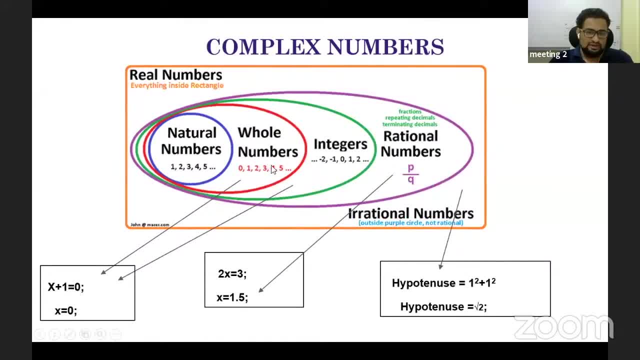 my problem. So I need to have 0 and also I need to take integers, which are negative numbers. So natural number, whole number and integers all together will help us in solving the equations- linear equations- to some extent. However, life is not simple, So in life there is a 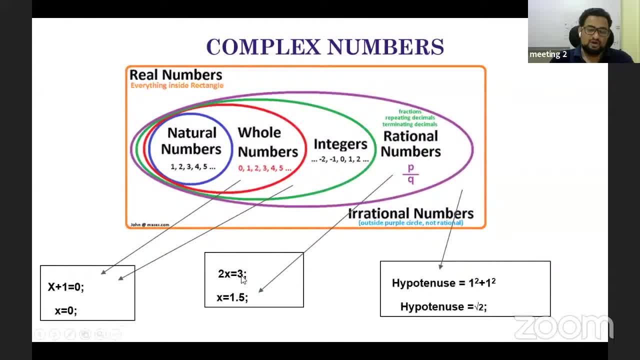 lot of problems. So, for example, if we solve the equations, we also come across 2x equal to 3.. So 2x equal to 3, the answer is not the answer to this. x does not belong to this set. 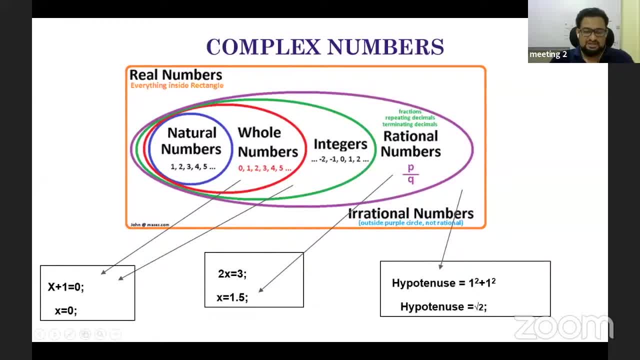 So then we need to. then the research, the mathematicians, they were motivated to find out rational numbers. So rational numbers are of the form p by q, where q is not equal to 0. So this gave rise to rational numbers, and I tried to find out the rational numbers. 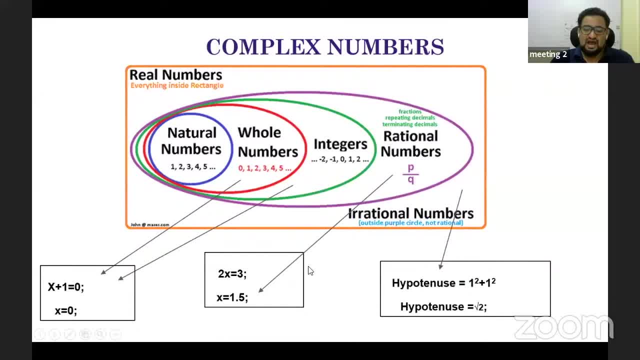 So I did. So I found out the rational numbers, So I found out the rational numbers, So I found out the rational numbers. so you can see that now the number, the our set of numbers increased here, and it is 1.5, is not a. 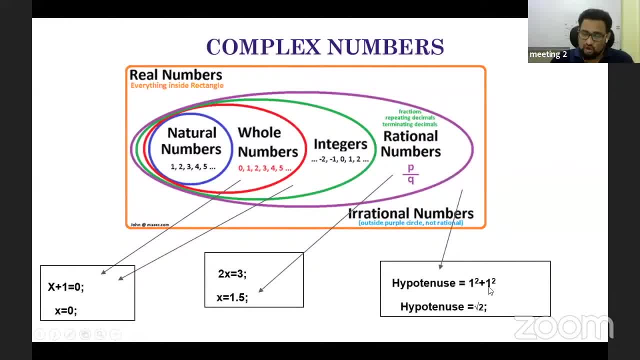 means the only rational number is not enough. in our real life we also, come suppose you have a triangle in the triangle in the both sides. uh, the adjacent side and the opposite side is made up of 1, 1. then hypotenuse is root 2. root 2 is not a rational number. root 2 is an irrational number. 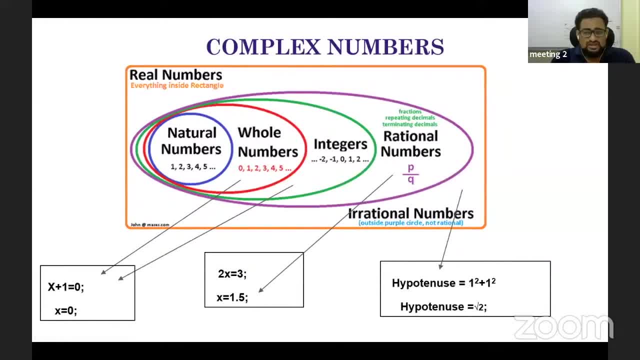 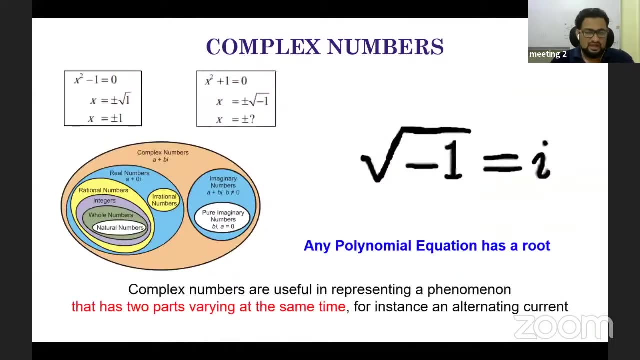 so now? so so both now, taking together rational number and irrational number, they form the real number. okay, so now, with this real number, we are able to solve the equations in real life to some extent. however, there is another problem. another problem is that if there is an equation of the form x square minus 1, equal to 0, the life becomes very simple. 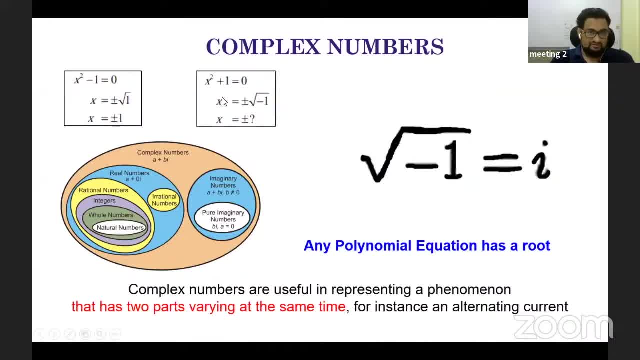 right, we get x equal to plus or minus 1. however, on the other hand, x square plus 1 equal to 0. life is not simple. we need- okay, we need to solve this problem. okay, we need to solve this problem. and how to solve this problem? uh, so the people thought of um means discovering or inventing new. 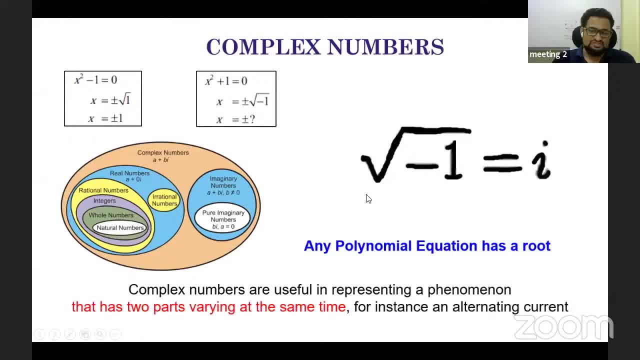 number, new number, which is the, which is called the complex number, which is the imaginary number. so now you can see that, this whole, you can see that complex numbers the first. i told you that the first story is that from the, in the real life we have to solve so many problems, but in that it is not possible to 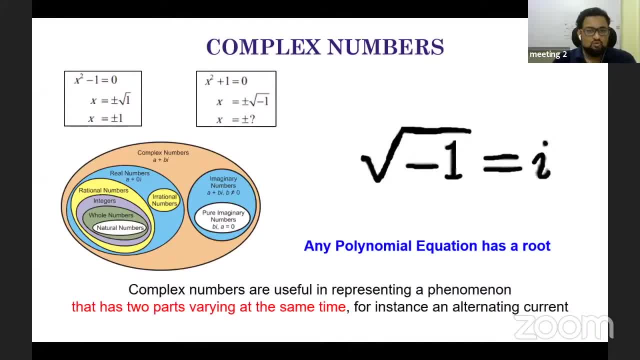 solve all the problems, okay, whichever is arising. so we need we, there was a necessity for us to invent a new number system called as complex number system. and then we had, we introduced this imaginary number system and then club together with real numbers where actually, if a plus uh, okay, it is a plus ib, where a and b are real numbers. 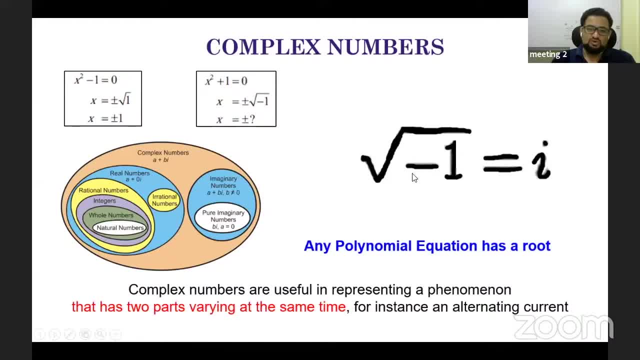 so this together gives the complex number where i is equal to root of uh minus square root of minus 1. okay now the first perspective which i told. the first story is that comp, you know the inter, the, the complex number was introduced to solve the polynomial equations. 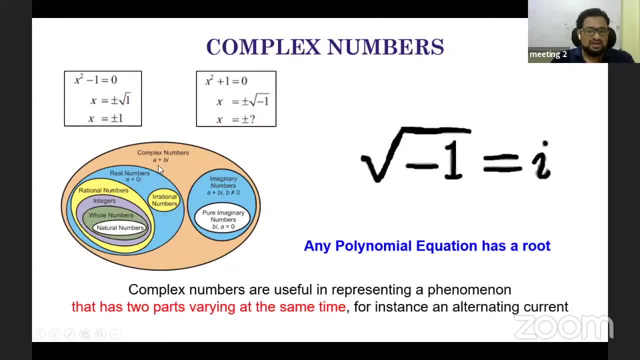 okay, okay, any polynomial equation has a root when you take, when you, because complex number can also be, uh, real numbers, like we'll see here. a plus zero i is also a complex number, right, so now, complex numbers are useful. so now, this is the story, that to make our life simple, to solve, 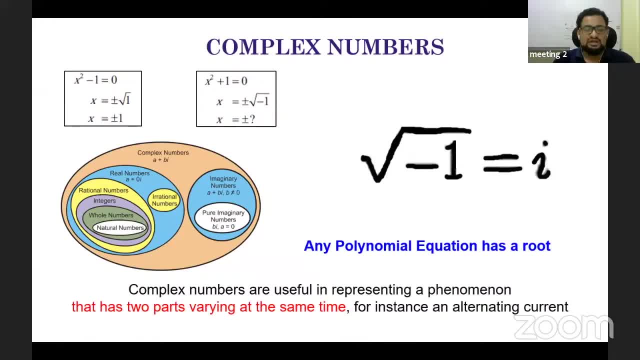 our problems, we introduce the complex numbers. now, coming to the second philosophical aspects of complex number, complex numbers are very useful in representing phenomenon that has two parts varying at the same time. please remember, please try to understand here, that complex numbers are used to represent a phenomenon that has two parts varying at the same time. 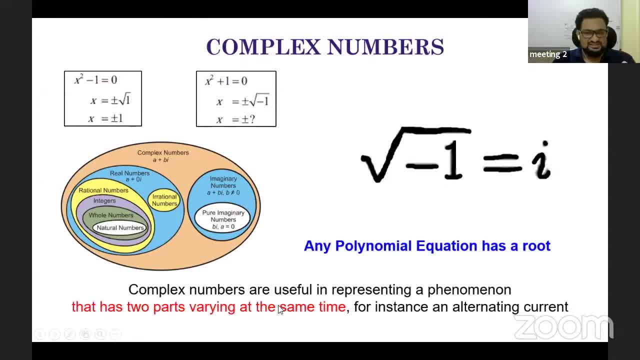 same time. okay, that means i, i have two entities, i have two entities which are real. however, i need to connect these two entities with some relation. right, with some relation. so that is the. that is the idea of complex numbers. i have some, i have some very interesting examples. the next slide. 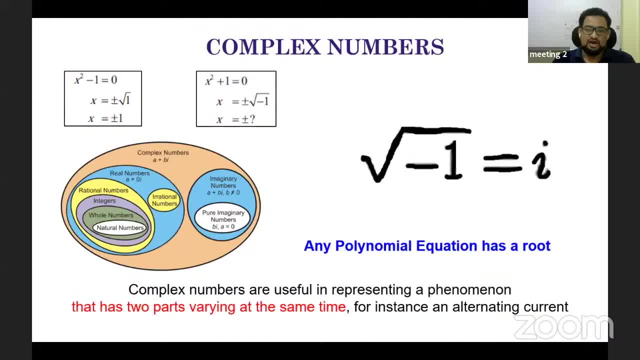 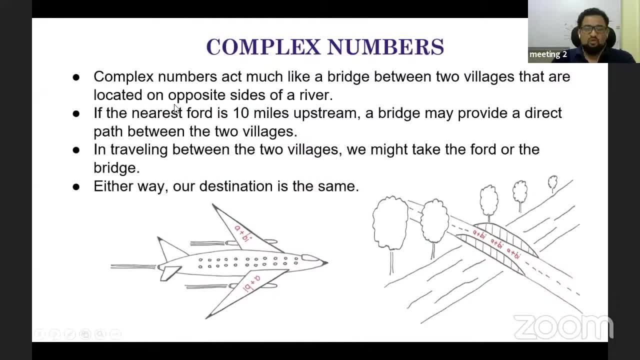 will make, give you a very philosophical idea of these complex numbers. okay, okay. the next slide says that: okay, complex number now. whenever you say that, okay, okay, now, let me, when you say the complex number, a complex number, whatever the operations which were, uh, which were applied on, 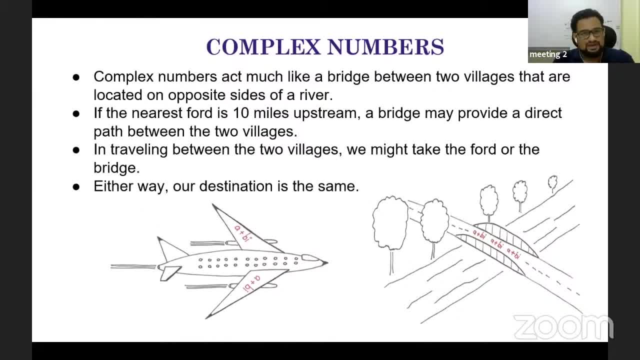 the real numbers, the complex number same operation can be applied. so complex numbers act as a like a bridge between two villages. suppose there is a village one. there is a village, say the there is a village one, there is village 2 here. okay, so there is, there are two villages that are located on opposite side of a. 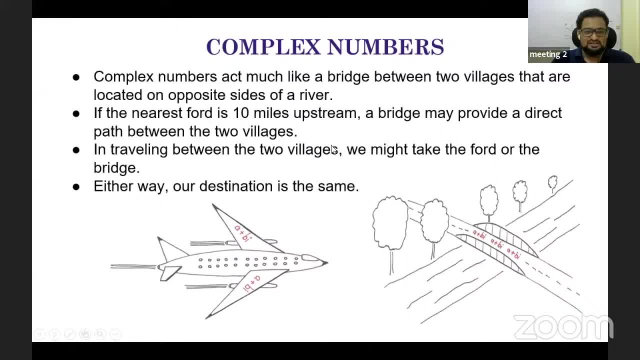 river. if the nearest, for that means if the nearest location which to reach the village is 10 miles upstream, means you have to see you have to go upstream and then 10 miles and then okay, then you have to reach the village 2.. so from village 1 and village 2, in order to reach, you have to cross. 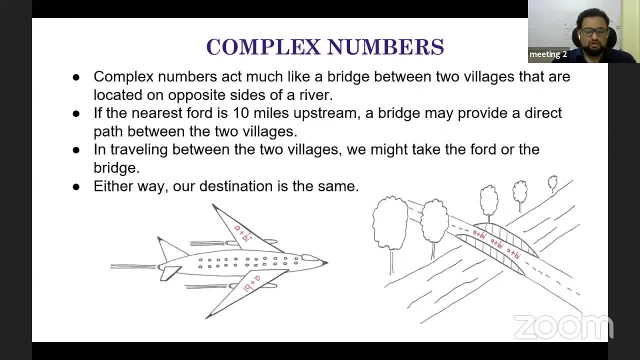 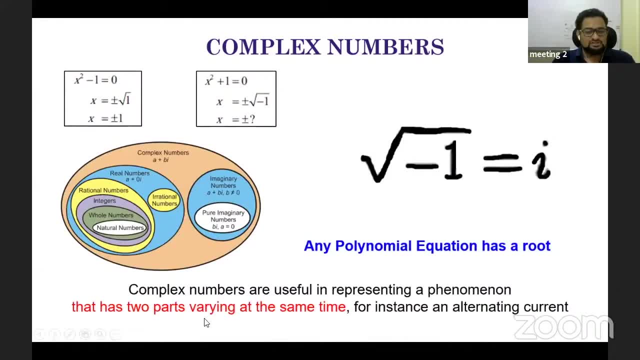 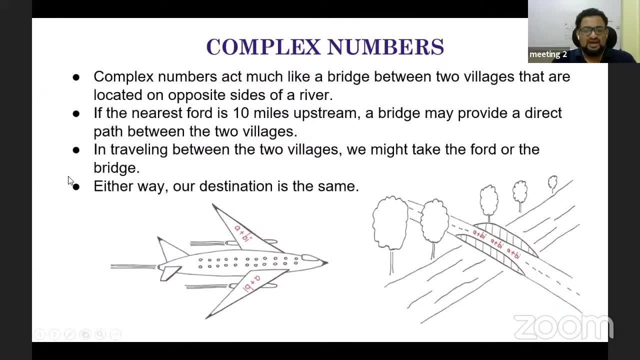 10 miles, okay, and then now there are two. this: these are two entities. please let us go to this slide again. complex numbers are useful in representing a phenomenon that has two parts varying at the same time. okay, so now i need to bridge these two villages with the help of a. 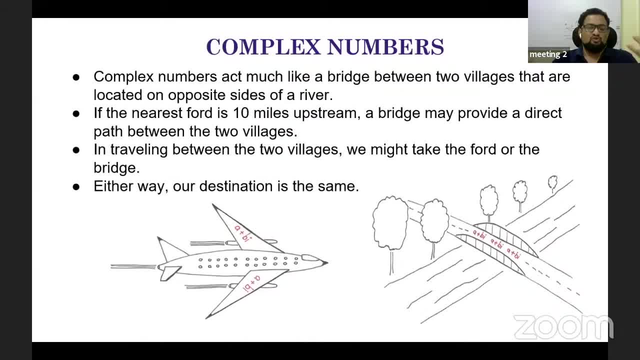 bridge. that is the complex number. so a is a village one, b is a village two. now i need to form. i need two, two villages, and this gives the philosophy of, okay, a plus ib, which is a complex number now. so yesterday i was discussing with my professor, professor sir, so he told me that 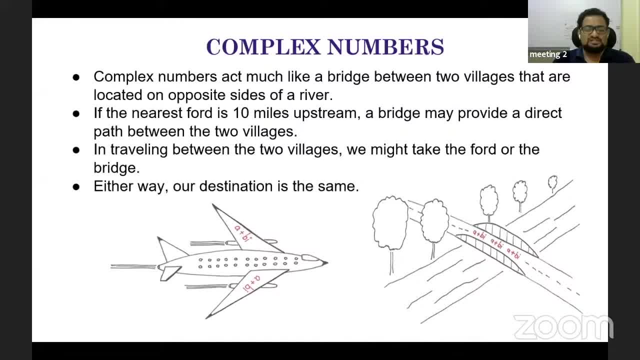 see this bridge. okay, now, why do you call this bridge as a complex number? the reason is that this bridge has magnitude. this, so any complex number will have magnitude. magnitude means modulus of that particular, so it is square root of x square plus y square. gives you magnitude, as well as there is a theta. 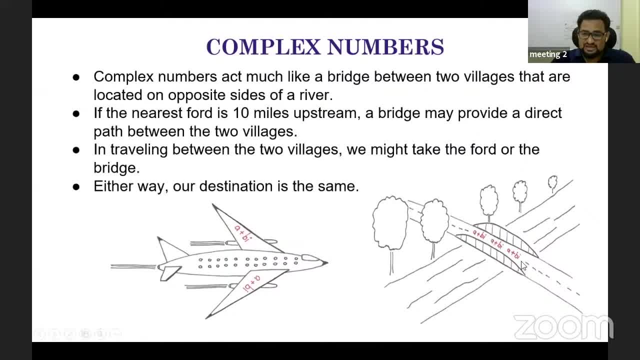 associated with a complex number. now, this number, okay, this bridge has- why it is called a complex number, because it has a magnitude- is it has a direction associated with this, with this particular bridge. okay, what is the strength of the bridge? what is the orientation of the bridge? so that is. 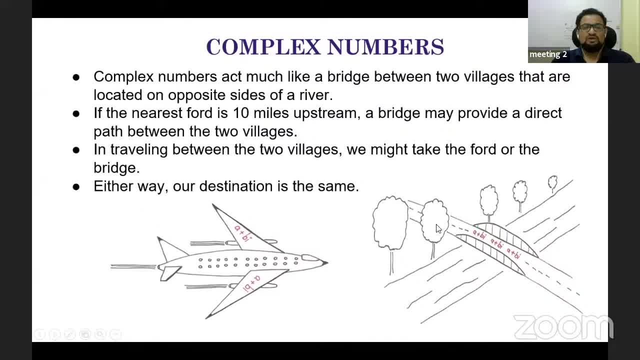 the reason this, this bridge between two villages, can be called as a complex number. okay, so in order to tell a complex number, there should be a direction, theta, and which is a tan inverse of y by x, and there should be a square. modulus operation means the length of the norm or length. 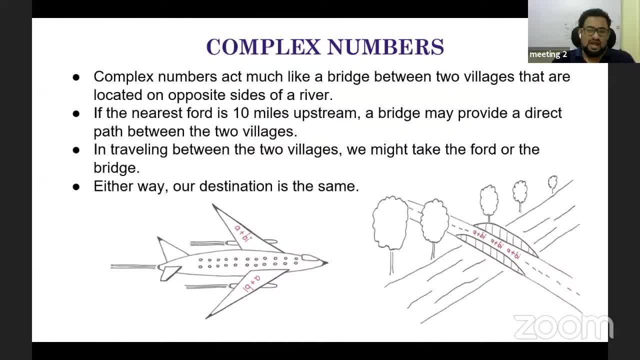 of the complex vector which is square root of x square plus y square, and similarly, same principle is used in applying in designing the wings of the aircraft. so there are two air wings of the aircraft, on the left side and the right side, whereas this body of the plane represents a vector. 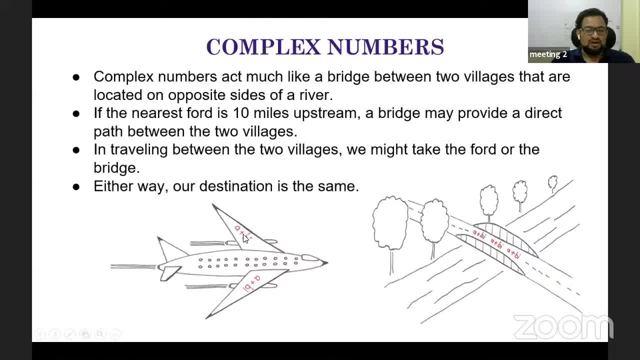 a complex vector where it connects the wing one and wing two. so that is how you can take it as a. so this body of the plane is, can be represented as a plus ib. so a plus ib, it has a, it has a magnitude, it has a direction. so we can tell that. complex numbers- okay, we use complex numbers to. 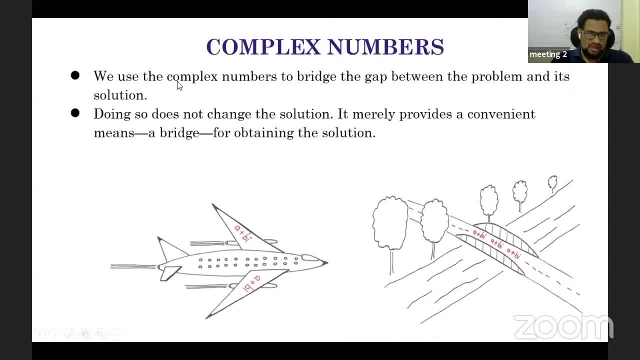 bridge the gap between the problem and its solution. okay, so we use complex numbers to bridge the gap between the. i think i already explained you that why. what was the need for the complex numbers doing so? uh, doing so does not change the solution. now, we should remember that. 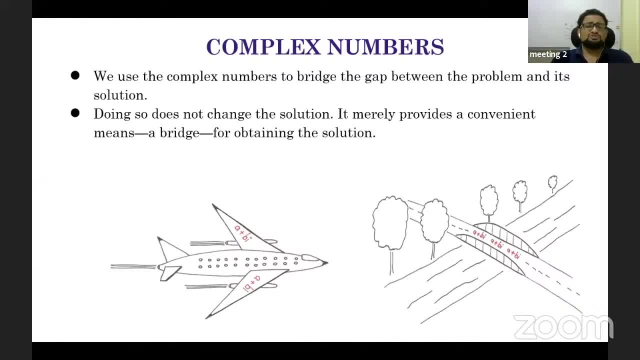 what i have done is that i have only bridged two numbers. okay, because those two numbers did not represent separately. i bridge two numbers, so now doing so does not change the solution. it is merely a convenient means of okay. means of uh, bridge okay. it is merely provides a convenient. 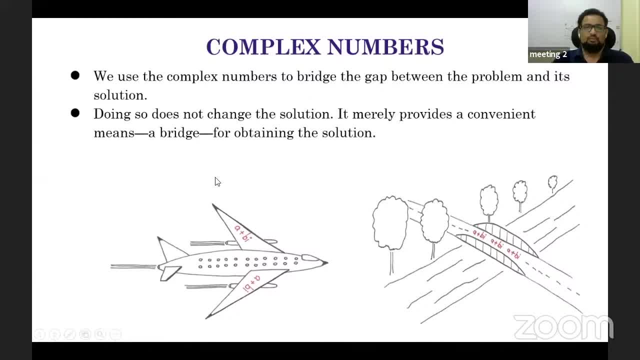 means a bridge for obtaining the solution. okay, i hope the idea of, uh, the philosophy of complex number is very clear. so yesterday there was a question when professor nagushen sir was giving me the lecture, that what is the real world example of complex number? i think this will. 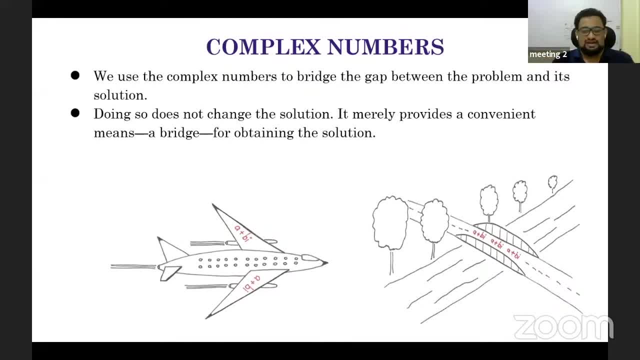 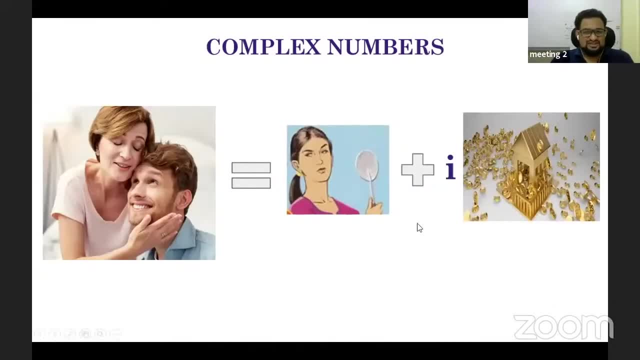 give you a very brief, very, very philosophical idea of complex numbers. i have some more examples, so this is a very interesting slide which i thought yesterday and then, okay, you miss. i created this slide today morning. see, this is mother-in-law, this is son mother-in-law. 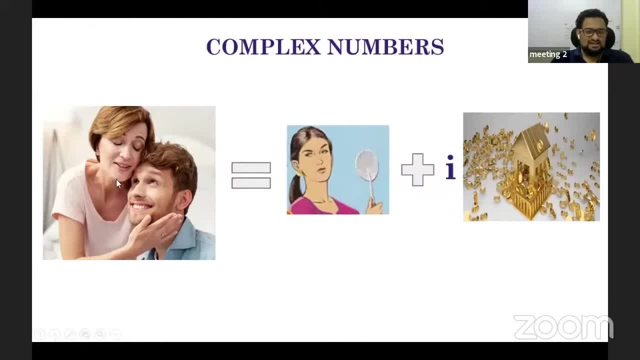 and son means the marriage of a marriage of a daughter daughter-in-law. okay, daughter-in-law is very much connected to the property or the wealth what the daughter-in-law brings. okay, so now this can be a. so mother-in-law is connected to the property or the wealth what the daughter-in-law 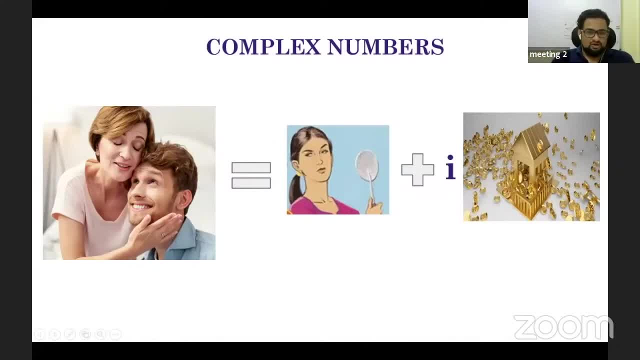 brings, okay. so mother-in-law, when she is looking for for a daughter-in-law, then mother-in-law is focused on daughter. daughter-in-law should be beautiful also, along with beauty, which is so. mother, daughter-in-law is real and whereas the the wealth she brings when she comes to the. 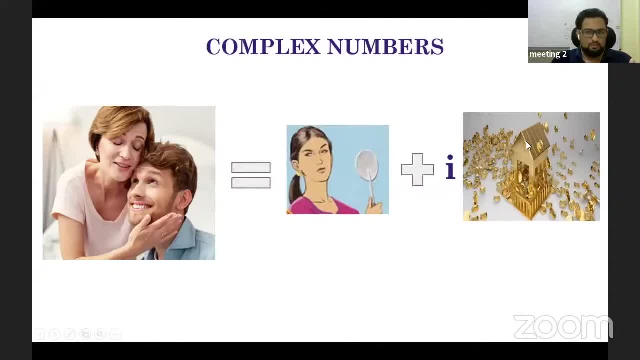 to her house with the as a daughter-in-law, she also brings some property. okay, so now this: i think the idea of complex number is very, very clear, that mother marriage is equal to our mother, mother-in-law m equal to daughter-in-law, plus i times the wealth, the property, what she brings, whereas you can see, 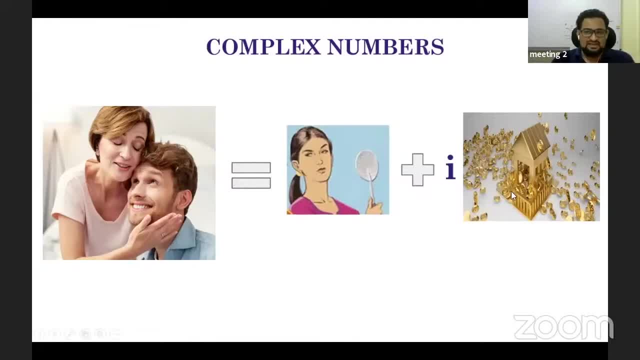 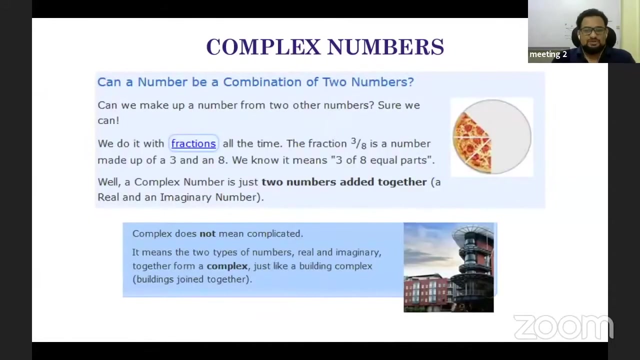 that daughter-in-law is real, whereas we, whereas, whereas this property is attached to daughter-in-law- okay, which is you okay. which is also attached to the mother-in-law when she is, when she is married, okay, so this property is a something which is, which is a imaginary way. you can see that. another example to make you. 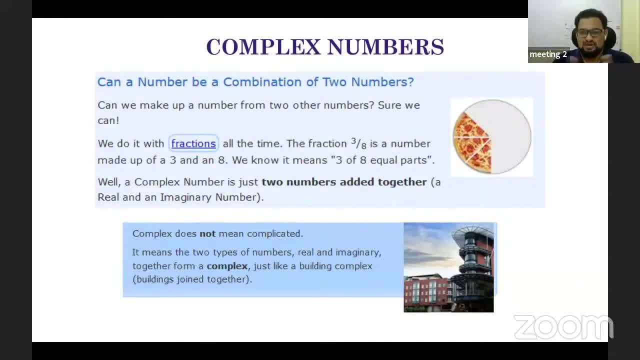 understand. i have tried my best to collect so many things to make you understand the complex number. so another way to see the complex number is: you have a pizza, okay, the pizza is made up of eight pieces. now can a number be a combination of two numbers? so so now, now my 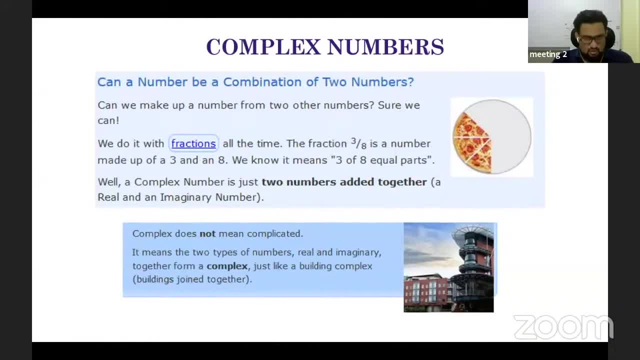 requirement is: you want to make a number for each of four pieces which are equal to or equal to a number. i want to make a number for each one. i give a number crian, we use so rotation- made up of 3 and 8.. So this gives you an idea that I am representing a number fraction. 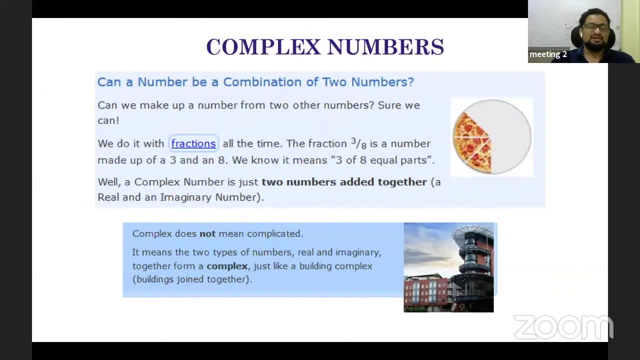 3 by 8, using two numbers. So I can say that I can. in a nutshell, I can say that 3, so I have to get one number, one entity, so that I have to combine two entities. So it is. 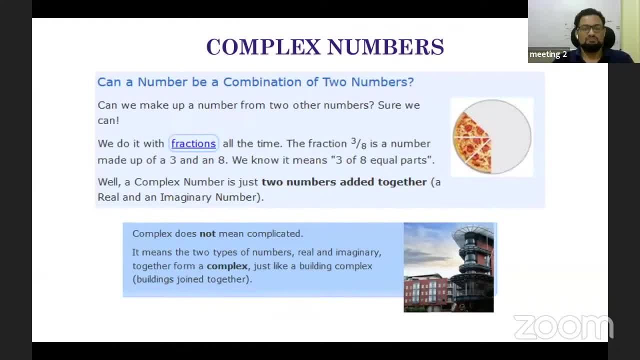 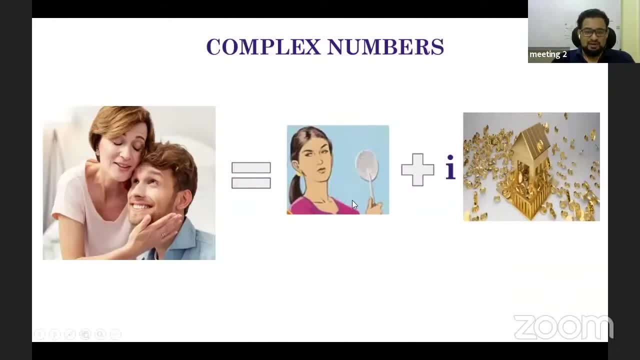 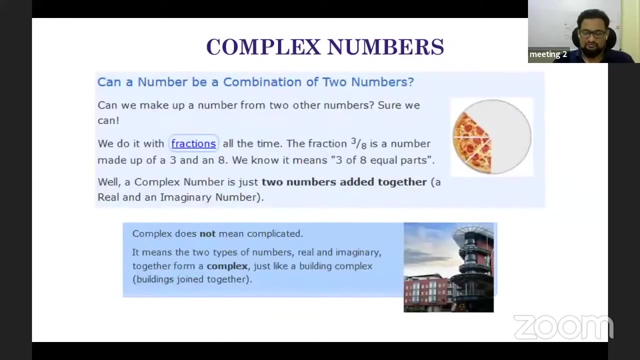 same thing. you can tell that a complex number is made up of two numbers And two numbers I am combining to make it as a single number. So same way here. two things. I am combining: daughter-in-law and money the property to for a marriage or for a for the mother-in-law. 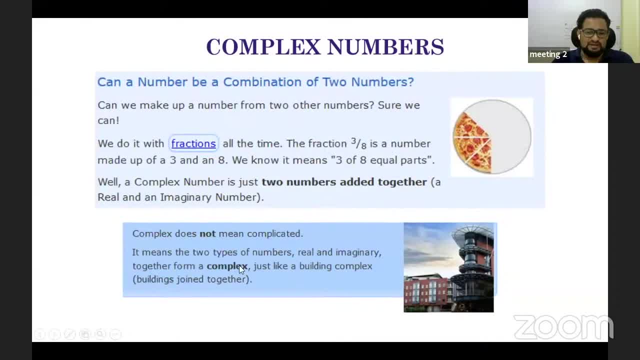 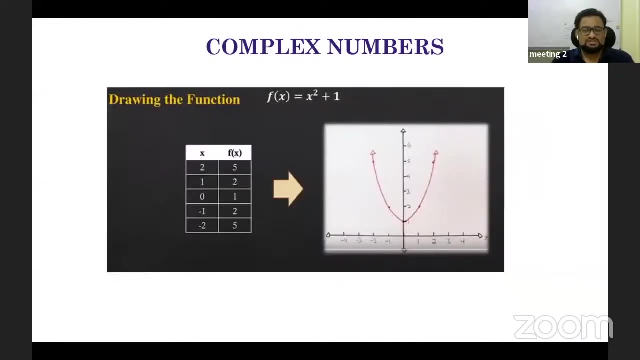 So like this. so you can see that it means there are so complex numbers are used in everywhere, Everywhere there is a relationship between two entities, we need complex numbers to model them. Okay, so this is an just just to show you that how f of x equal to x square plus one. 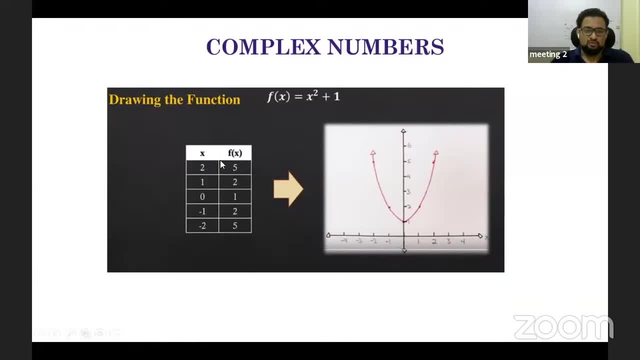 graph will look like. Okay, now, when you plot, when you start putting the values into x value as 2,, 1,, 0, you can see that you will get a one graph, but when it is 0, the graph does. 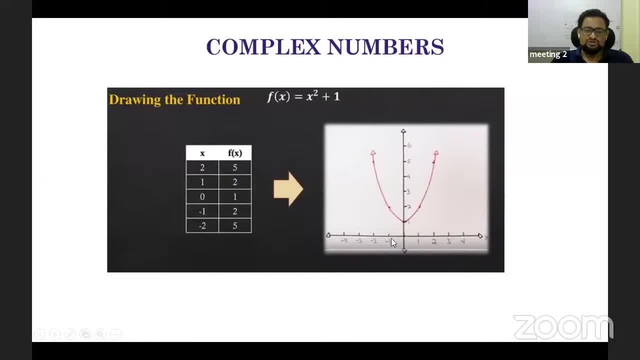 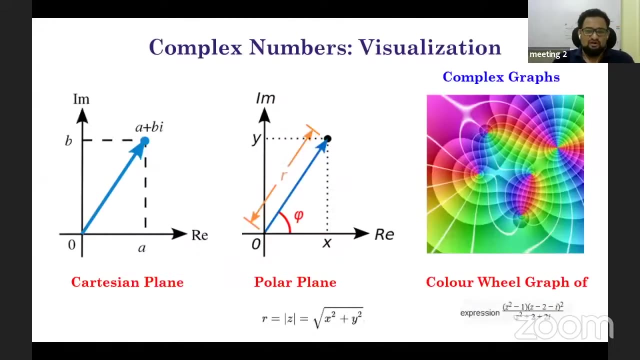 not touch the x axis. That means, for 0, there is no solution here. Okay, for 0, there is no, no solution on the real axis. So this is one way of mathematical way, of our visual way of looking into these complex numbers. So there are. I am in the literature I have 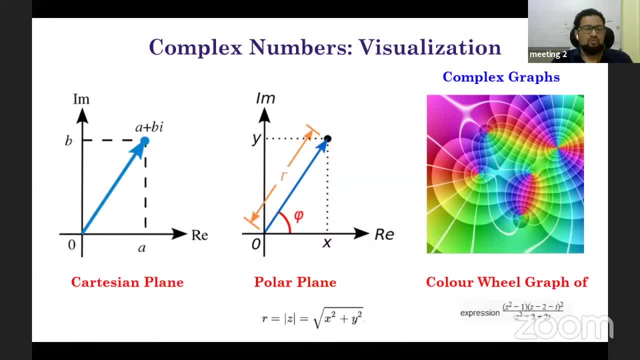 found out that there are three ways to visualize the complex numbers. One is the Cartesian plane. Now I give you the example of a plus bi. a plus ib is: it has a, it has a magnitude and it has a direction and all the operations which can be done on real numbers can be done. 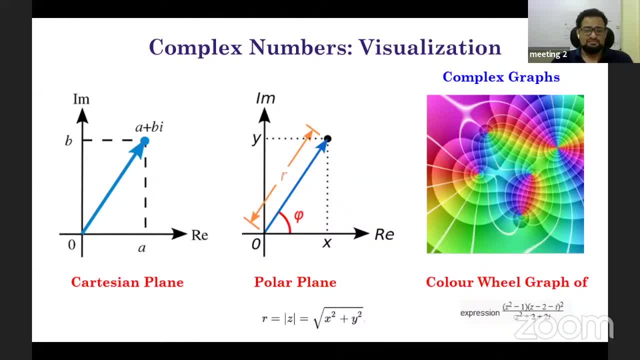 on this particular, this complex numbers. Okay, the other way of representing is is using the polar form. Okay, So this is the real numbers. this is the linear numbers. Guess, I find this is because we have a little Plato. there are a lot of mansions in the form of: 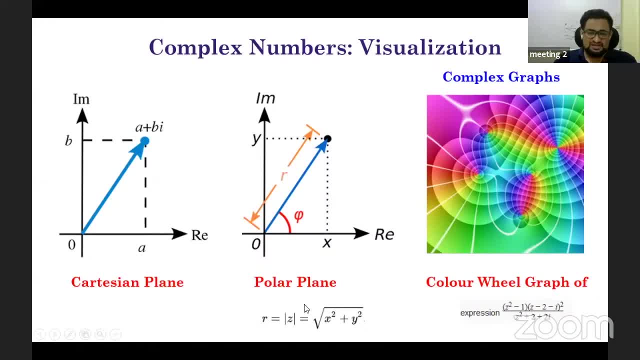 polar: x equal to r cos theta, y equal to r sin theta. okay, so r is square root of x square plus y square. this is the another way of representing where x is real axis and y is imaginary axis. okay, so now imaginary axis is same. okay, the imaginary axis. you can take the here. the value is 1 here. 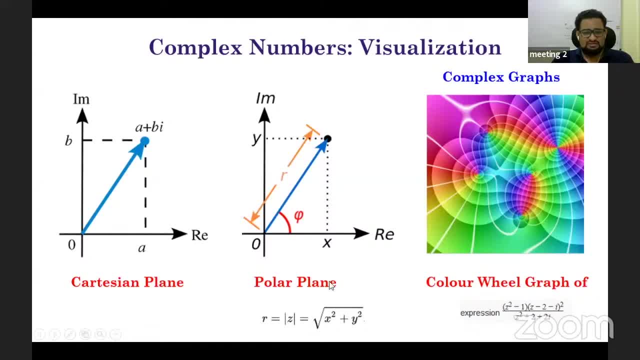 the value is minus 1. the here the value is i and the bottom the value is minus i. so another way of representing the complex number, see it is complex numbers are made up of two numbers. so i have gone through the literature and people have said that it is very difficult to visualize the complex. 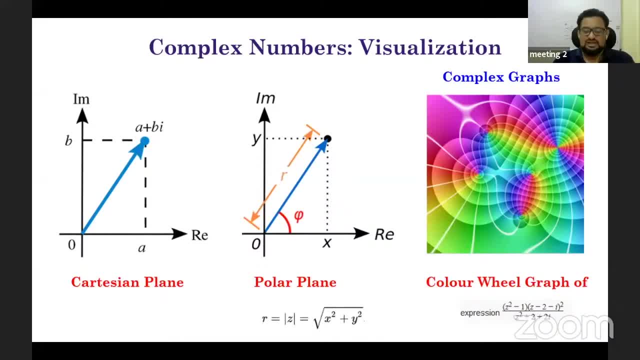 number in 2d plane. okay, in this visualize the picture representation of complex graph within 2d plane and we need require 4d plane to visualize this one. so people have tried to generate color wheel graph. okay, they now see. this is a color, this is a. 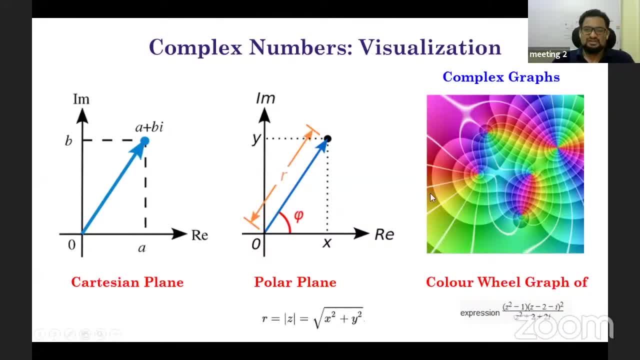 complex number and we need to visualize it in 2d plane and we need to visualize it in 2d plane. complex. this is a very visual representation of a complex number with colors, different colors. so now we you can see that here each color represents an one particular entity. okay, and we see that. 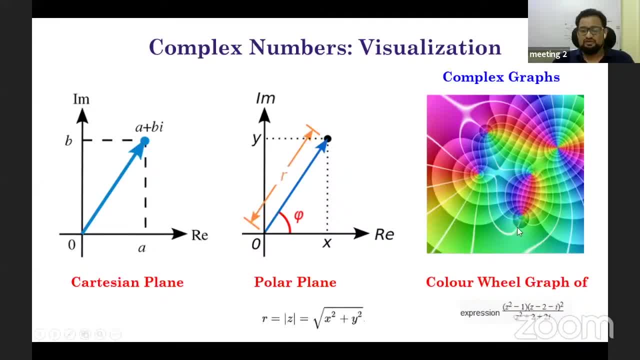 different colors are combined and this produces a very different, very beautiful art and yesterday's lecture we have seen that professor said that this is very wonderful. this is the in nature also, we find these colors and we can see that this is a very beautiful color and we can see that this is. 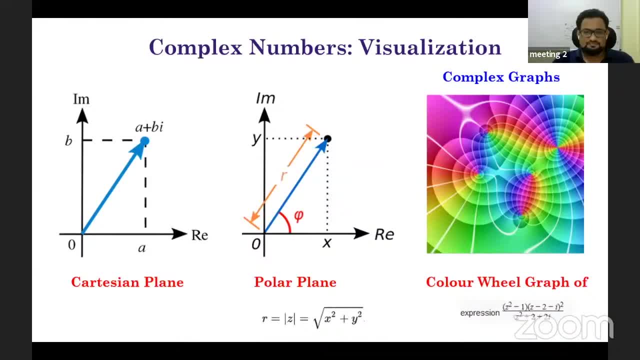 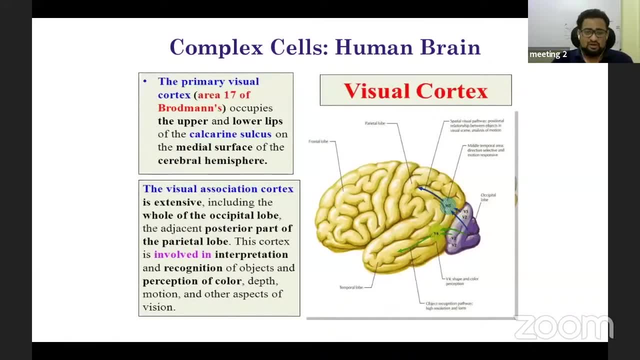 is a very beautiful color and we can see that this is a very beautiful, complex art. okay, so, and also, recently i reviewed one research paper for the journal of pattern recognition and in that i also read that. so that is the reason i brought this slide here. okay, another way of looking at the complex number is the. is the actually the complexity of, uh, cells? 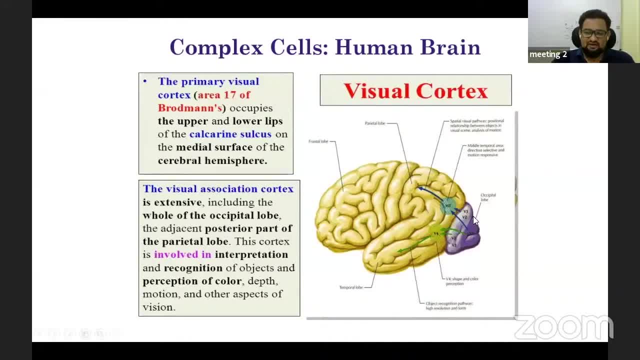 in the human brain. okay, so visual cortex is the area. okay, back portion of our area means the brain, which is responsible for wenig or complex activities and some for milliillion. this would be marginal in the 유нов but also should be easy to connect to. 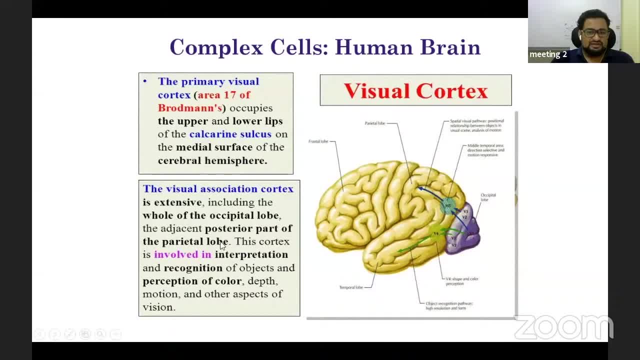 responsible for doing all kinds of operations, like it is. it is involved in interpretation, it is involved in recognition. i told you in my first few slides, i told you that cognition and recognition. so this is the part of the brain which helps you in learning features and also. 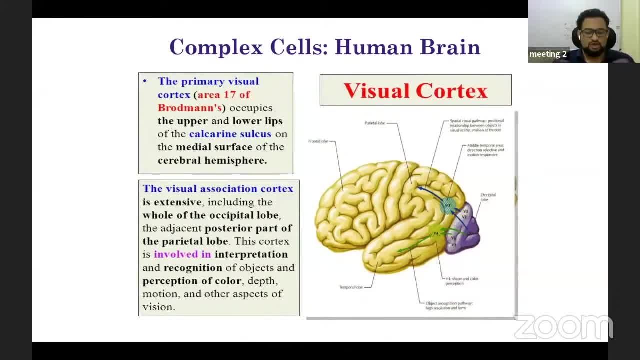 recognizing the, the person or the object. so the reason is that here, this part of the brain is made up of very complex cells. okay, where, where, where we can relate the uh, what you call. where, where we use uh, the complex numbers. okay, we can use complex numbers to uh to represent. 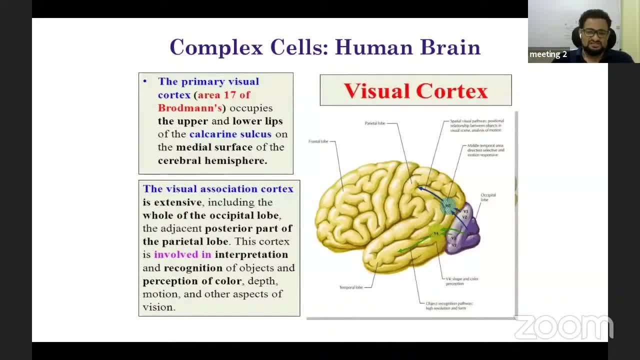 the signal which is generated from these cells. so this is one, one example that our human brain also uses the complex numbers. okay, so i'm not going deep into that because of shortage of time, so you can, if you're interested. you can go more into the detail of this. 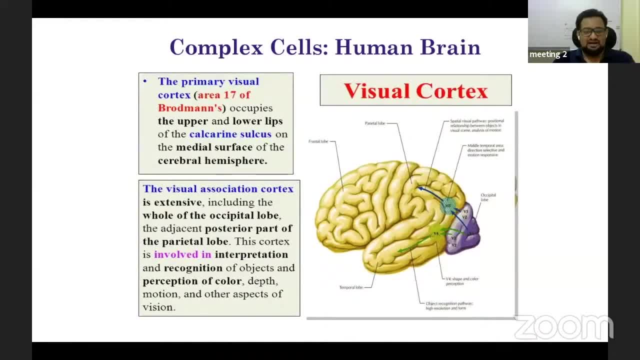 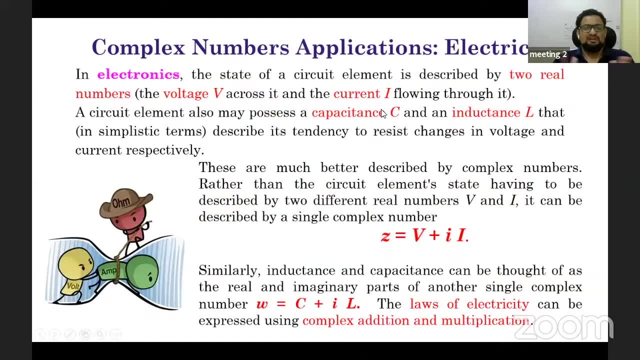 particular part of the brain, so i'm not going deep into that because of shortage of time- particular thing, and that research paper had cited, uh, this idea, so i thought that let me bring it here. and so the other very famous example: see, whenever you try to search about a complex number, 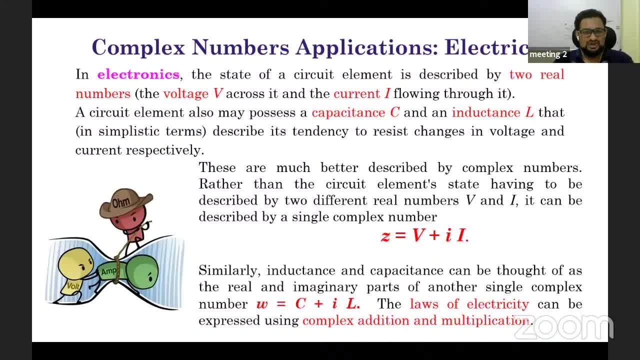 in the internet. this is the first example which you try to get it okay. so they try to explain you. complex number with a with an example of a current. so a current is made up of voltage as well. means a: a circuit is made up of voltage as well as the current. 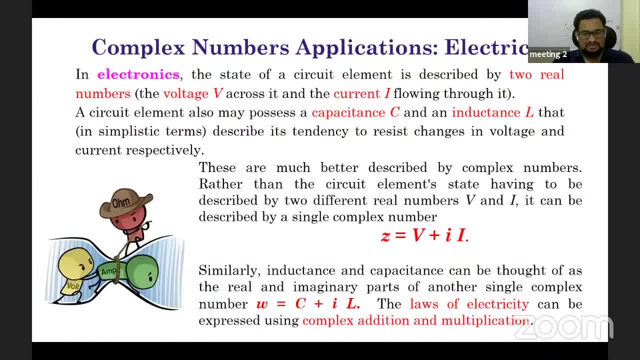 okay. however, voltage and current should go together. they are not as separate entities. so i represent these complex numbers as this: voltage and current as z equal to v plus i. and now you know that same operations which are uh, applicable for the real numbers, are also applicable for the. 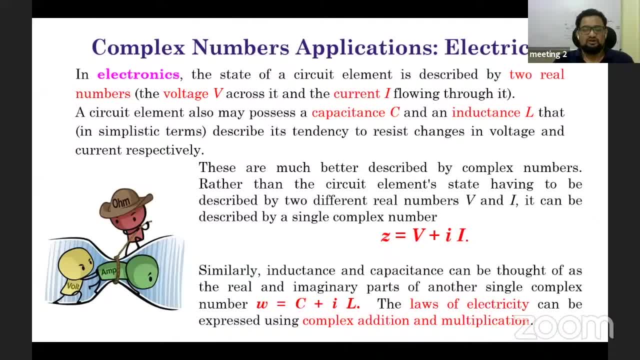 complex numbers. so now i can do so. so many kind of multiplication, addition, all kinds of operations i can do. similarly, the capacitance and inductance they are now, they are now coupled together as a complex number. okay, see, in the same manner, you will be okay. this is the second. 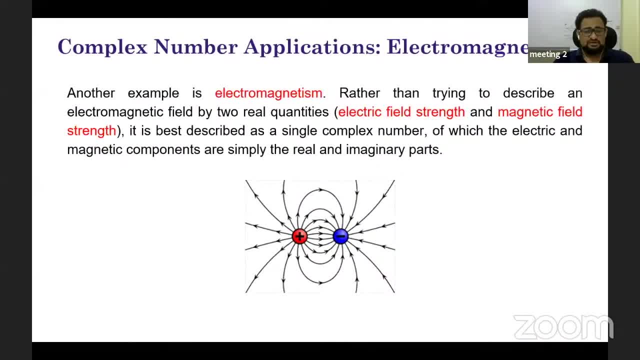 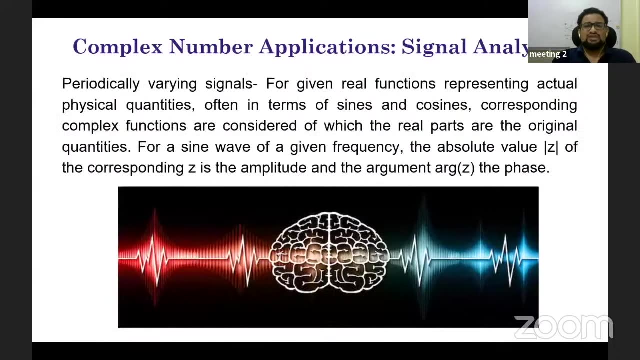 most famous example for complex numbers which, if you try to search in the, excuse me, so, um, if you try to use electromagnetism, in the electromagnetism, electric field strength and magnetic field strength both go together, so they need to be combined as a complex number, right? so there are many. 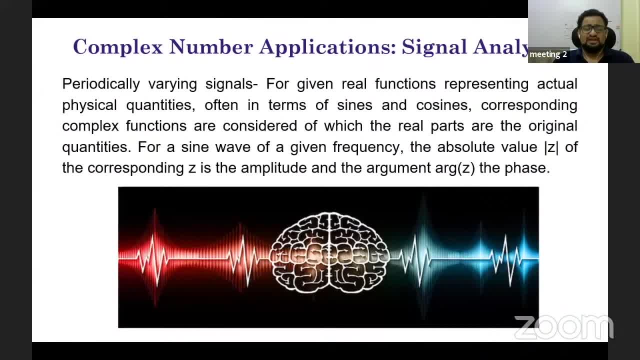 uh, i think they- i have already explained this. um, okay, in different phenomenons, different, different, different signals in the brain. okay, uh, signals in the brain are very complex, okay, and uh, they need to be represented using the uh complex numbers. okay, so so in future, because of more automation, digitization, so it is more more complex number is going to. 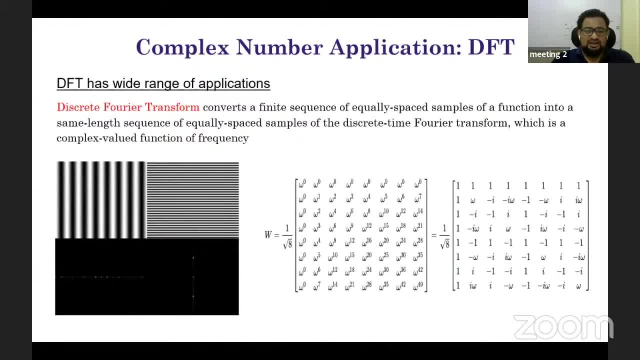 be used in that particular scenario. another very important, very famous example of complex number in the signal processing area is discrete fourier transform. so discrete fourier transform which converts a frequency se- sorry, a spatial domain signal, a spatial domain, converts a signal from a spatial domain to the frequency domain. okay, now you can see that there is a. so this is. 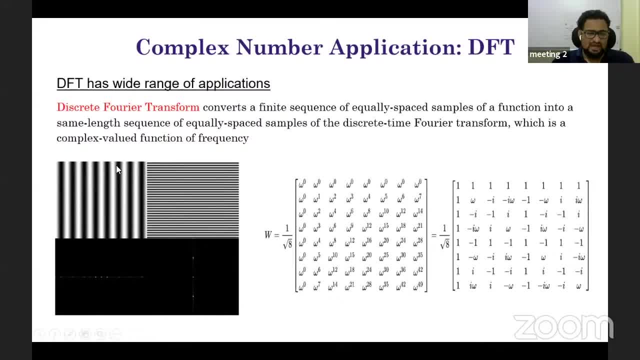 this is a frequency example- sorry, this is a spatial example- where the signal is becoming positive or negative. positive, negative if you take black as a positive. so this is a signal which is varying. similarly, this is another signal which is varying now, when you plot this signal in the frequency. 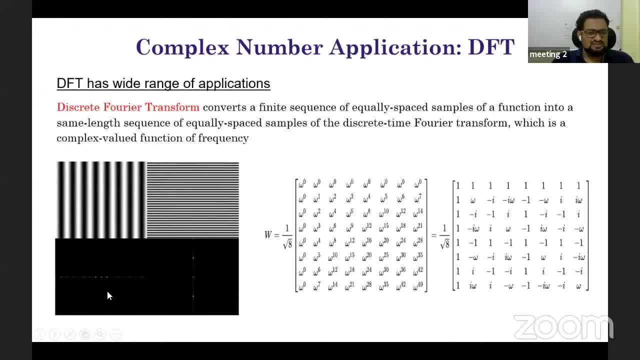 domain or Fourier domain. you can see that this entire image is represented as three dots here. Okay, so these three dots represents three types of frequencies, right? Similarly, you can see that this is an. these lines are modeled as three points in the frequency there. 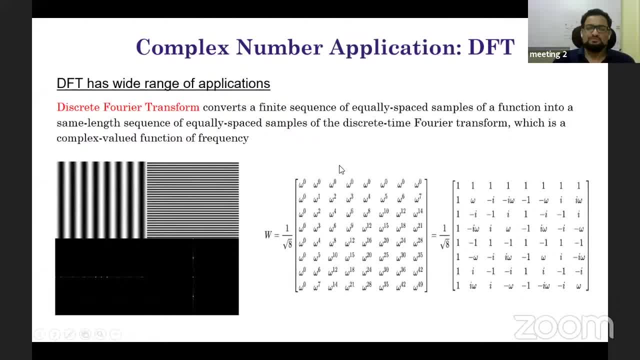 are of the three kinds of frequencies which are more So. this is a very famous Okay. so now the question is why to convert from frequency to spatial domain, to the frequency domain, So in frequency domain, like, for example, a problem of noise removal, a problem? 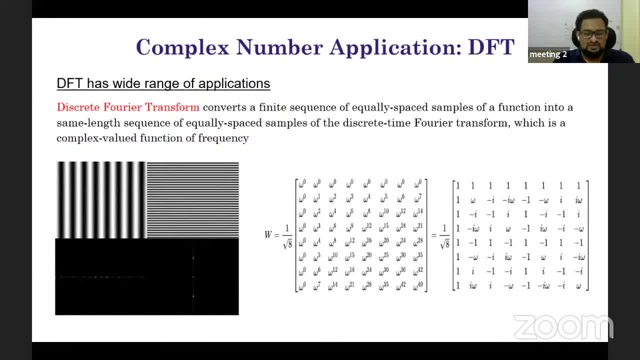 of noise removal is not possible means it becomes very difficult in the spatial domain, whereas in frequency domain the problem of removing the noise becomes a very simple. so so the concept of transformation from one form to the other form, and now the main driving principle behind this Fourier transform, is a complex number. Now you can see that I have 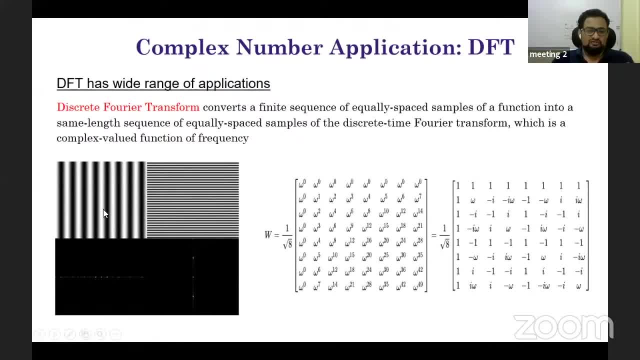 already written this diagram, This matrix. this matrix is used to convert spatial domain into frequency domain. Okay, this matrix is used to convert from frequency domain, spatial domain, to the frequency domain, And this is the matrix which is most popularly used in the JPEG compression. Okay, I have. 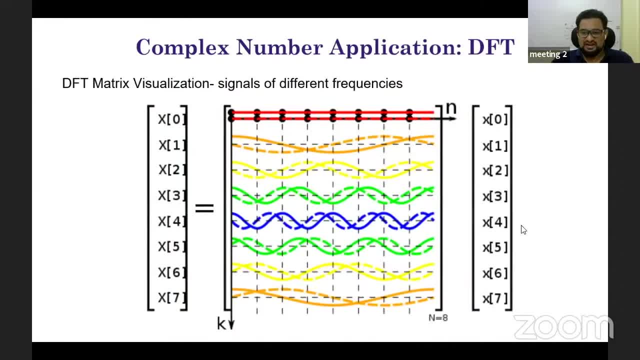 so now, just to make you so, these are all numbers, right? These are all symbols. Now I'm giving you a pictorial representation of signal. See, this is the, this is the signal, This is the DC signal. that means there is no fluctuation here, right? This is the direct current, Whereas 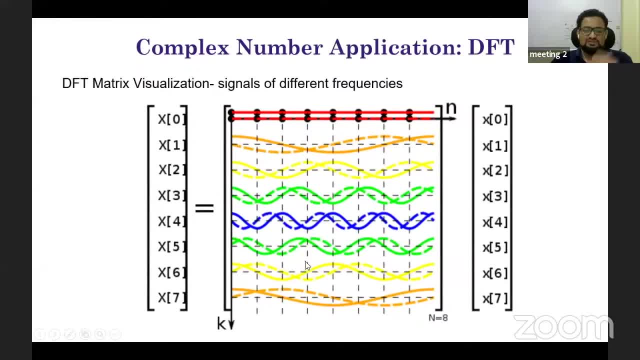 these are the alternating current. Okay, these are alternating current with different frequencies. So this is the visualization of this particular 8 into 8 matrix. Okay, So now what are the application of this discrete Fourier transform to discrete Fourier transform? you can see: 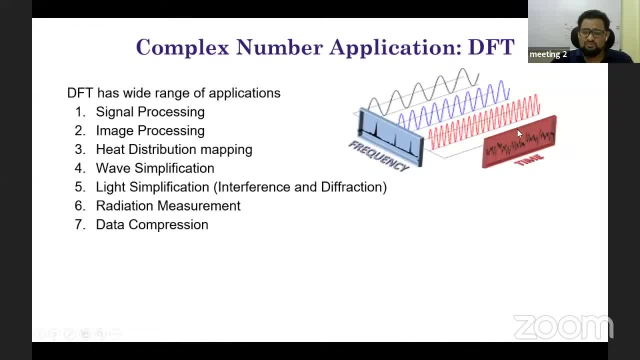 that different freak. you are modeling the time, you are modeling the signal into different frequencies. Now, lots of applications in signal processing: image processing, heat distribution, wave simplification, light simplification, radiation measurement, data compression- you can name any field everywhere. actually, DFT is used because, okay, because DFT is very close to 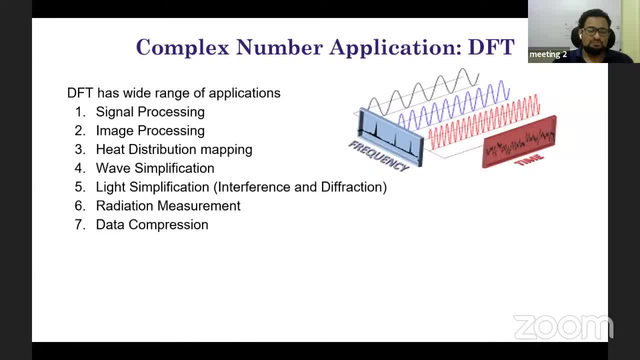 the human life. okay means, like human being, communicate with signal. my voice is communicated to you as a signal. my face is communicated to you as a signal, right, So similarly, my heartbeat is a signal okay. similarly everything, everything in nature. 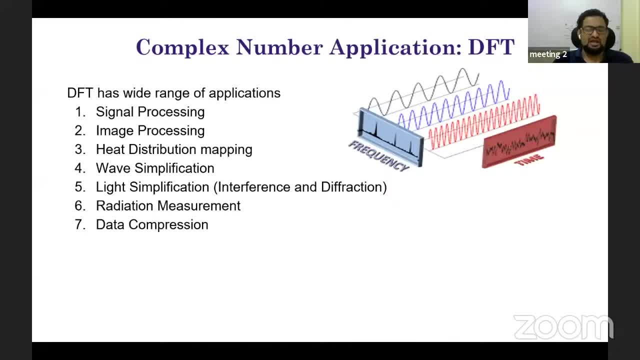 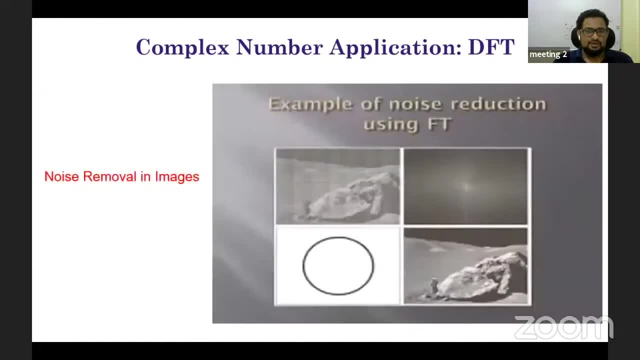 is a signal. So we need to learn from the nature and model it okay. so we need to model all those things okay in the real life. So another example which I want to show you is that discrete Fourier transform like for: 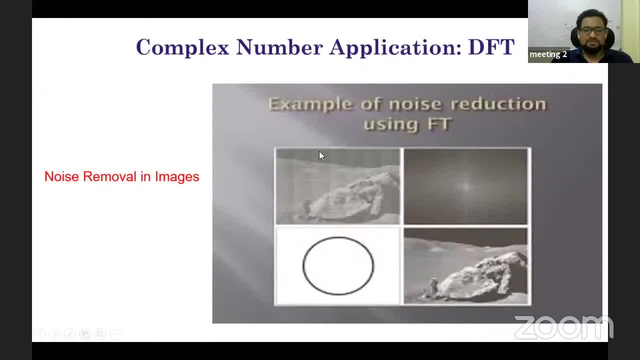 example, this is the image. I think yesterday in Dr Pradeep Kumar talked about this one like how to remove the noise like this is an image of the moon or Mars, I do not know exactly. So this is a moon, this is an image which was captured by the moon mission and then 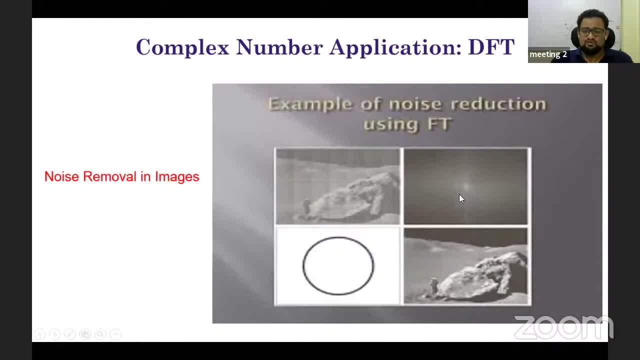 we can see that when I convert this image into frequency domain, you can see that this pattern, which was a, which was a noisy pattern, it is just a, some symbol. okay, just some frequency. Okay, I use this frequency domain filter and I try to remove this noise. 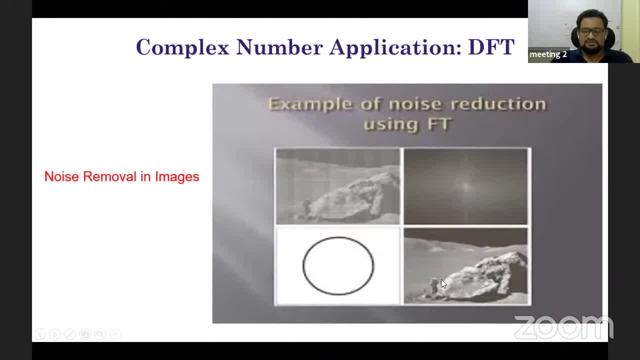 So you can see that this particular regular pattern is being removed from this particular. So this is application where discrete Fourier transform. So now the idea is that Fourier transform is driven by complex number, and that complex number is now helping us to solve different kinds of problems. 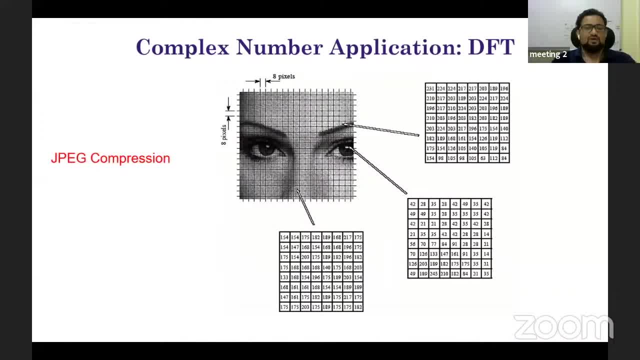 So another very important problem is JPEG compression. Okay, I have 15 more minutes So I would be a little bit faster. So JPEG, So JPEG compression is a very popular compression algorithm. I already have given you one example there. 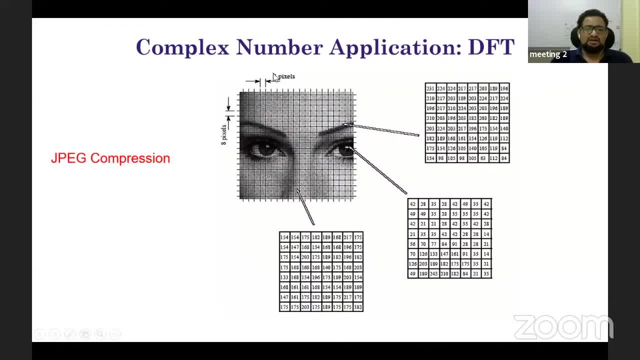 So JPEG compression uses 8 into 8, okay. it compresses the image by dividing into 8, into 8 blocks, 8 into 8 blocks again. this JPEG uses discrete Fourier coefficients: okay, discrete Fourier coefficients, Okay, Javed. 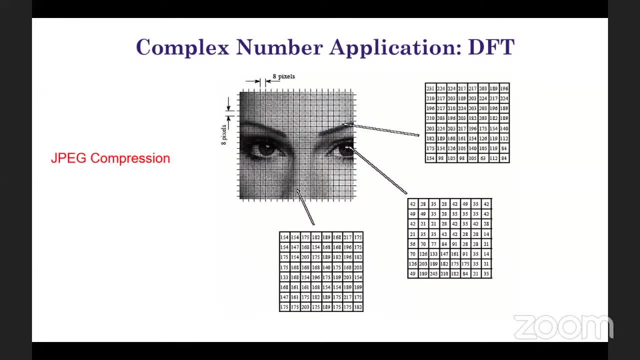 Ma'am. Hello. Yes, ma'am, Sorry for interrupting. Javed, You can take your own time. If you need additional time, you can just Okay. okay, okay, ma'am, I will just come, I mean. 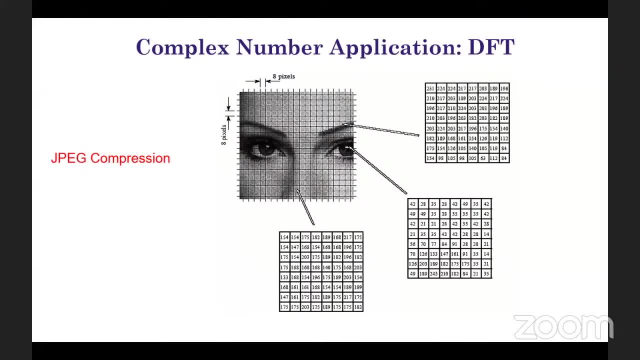 I will try to give as much as inputs, ma'am. Okay, Yeah, yeah, Thank you, Thank you. So this is a JPEG compression. You can see that a lot of, okay, a lot of- See. I'm not going to explain you in detail, but my whole intention of this slide was to 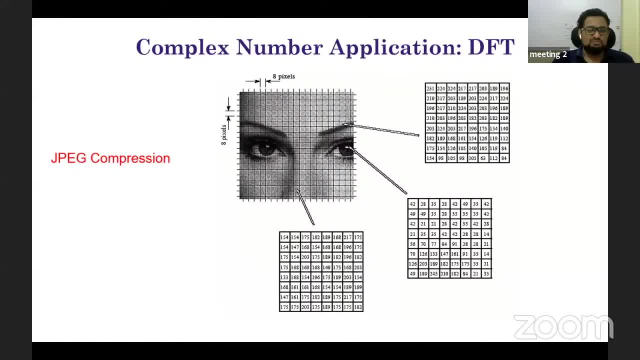 tell you that discrete Fourier transform drives you the most important application of JPEG compression. Okay, So I take the pixel and then I multiply that mat, this pixel, this 8, into 8.. So this 8 pixels is multiplied with the, with the coefficients, DFT coefficients, and then you get the different frequency, what you call. sorry that this is this matrix. it gets multiplied with this matrix, okay, with this matrix, and then we generate coefficients, and these coefficients are called the Fourier coefficients. 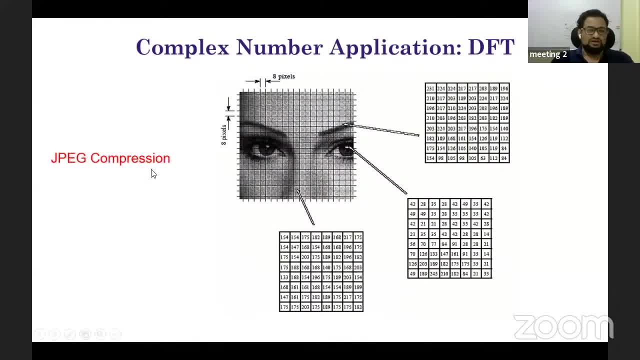 And in case of JPEG, it is not directly Fourier transform because JPEG uses discrete cosine transform. It does not use, It does not use sine wave because- see the main idea, the main idea behind the usage of cosine transform in JPEG is that 0, 0 value, the value of cos function at 0, 0, is not 0. 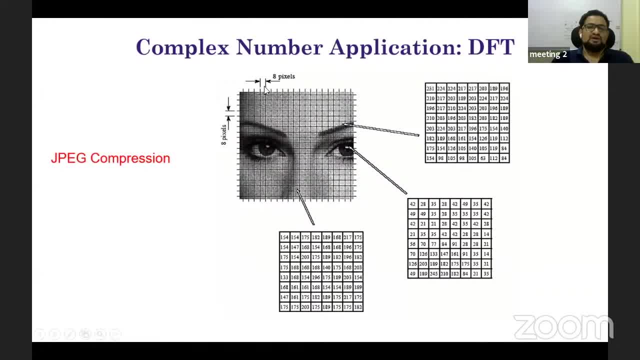 Okay, Cos of cos of 0 is 1.. So that is why see the most important signal in JPEG compression or discrete Fourier compression. So that is why see the most important signal in JPEG compression or discrete Fourier compression is actually the direct current. okay, that is the DC value. 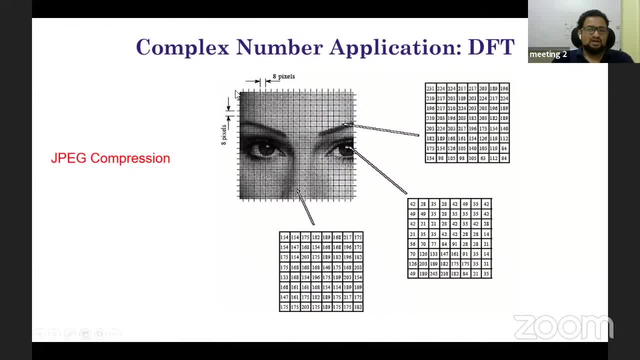 So if you use sine value, what happens is that you are going to lose the. if you are using the sine sine value, okay, sine transform. sine transform will not give you DC current, because sine of 0 is 0.. 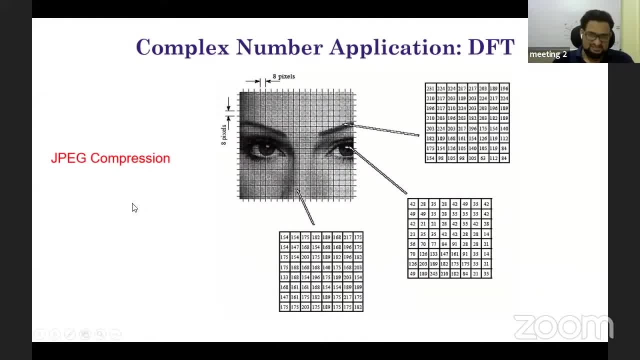 So JPEG compression uses discrete cosine transform. okay, discrete cosine transform for compression. So if you go through in the in the literature, you can find a big formula. So if you go through in the literature you can find a big formula based on this JPEG compression- okay. 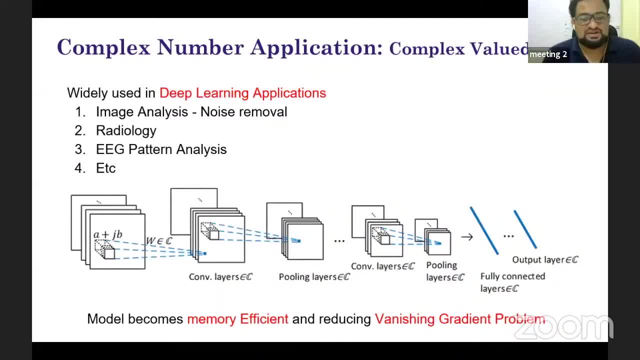 So now coming to the recent state-of-the-art literature. okay, now a very important application of complex number which we, being in the area of machine learning and deep learning, have found out that now people are trying to use complex numbers in deep learning. 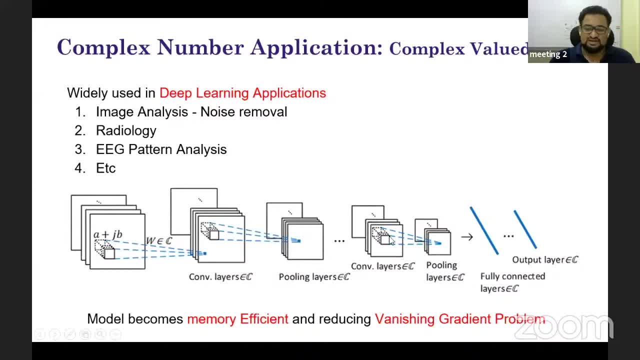 So this is see, this is this is a very I have reviewed, I think, that brain image which I have, which I have put Okay In my slide. that image has been taken. okay, that idea, the paper, actually the research paper, proposed a complex number for removing noise from an image. 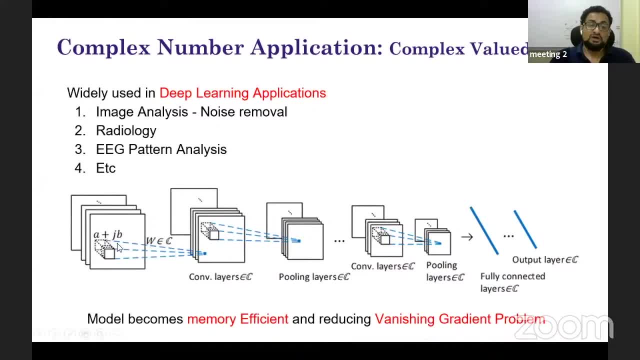 Okay. So now people are now moving towards using more and more complex numbers, because we know that complex numbers is not just one number, It is a. it combines two important components together and it tries to give you the brief means, tries to give you. 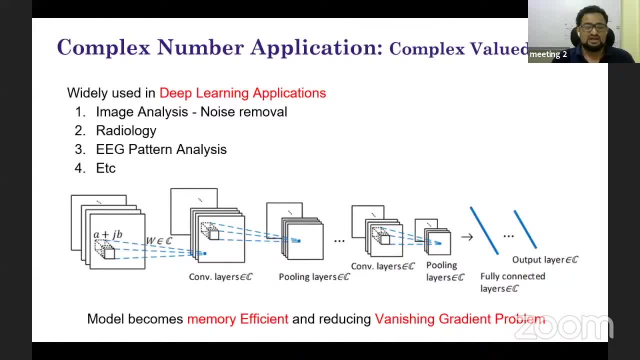 the feature. extraction, modeling and all those things are possible. So complex numbers are used in image analysis, noise removal. they are used in radiology, like, for example, they want to analyze where the bone fracture is, they want to analyze where the tumor is all. 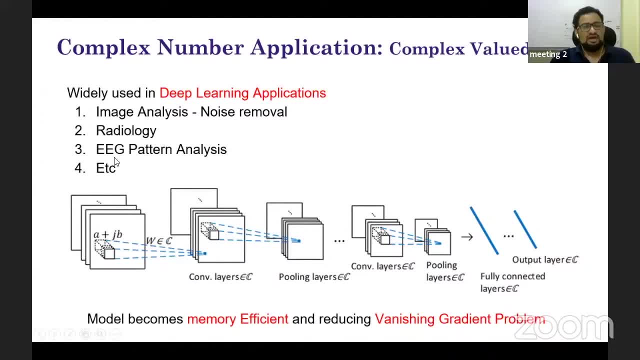 those things are possible using the radiology. And then we have EEG pattern. So EEG pattern also uses complex numbers for analysis. Similarly, you have, if you go through the internet and Google it, you have, tremendous applications which are actually see. I am telling you this: 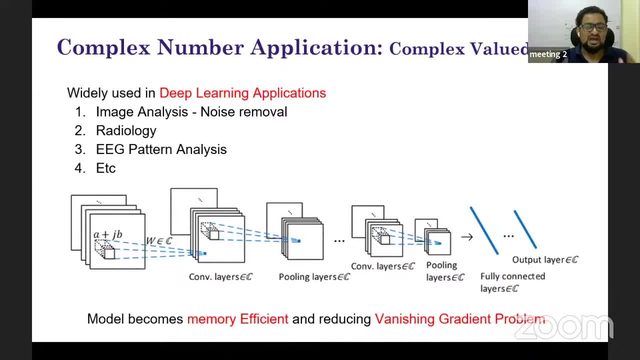 is the state of the art? deep learning models or the state of the art models in today's machine learning? in whatever automation you tell, they are the state of the art. and now the usage of complex numbers is giving them a new dimension of research they are getting. 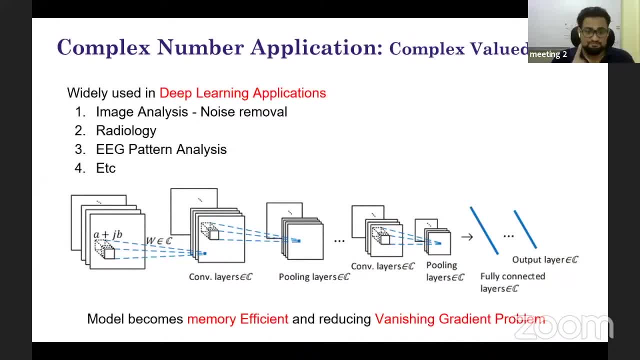 more accuracy and all those things are possible. And one more very important thing- I was just forgetting it to mention that the complex model, the complex number model, is more memory efficient and vanishing. gradient problem is solved, Means it reduces, because if you are gone through deep learning you will see that 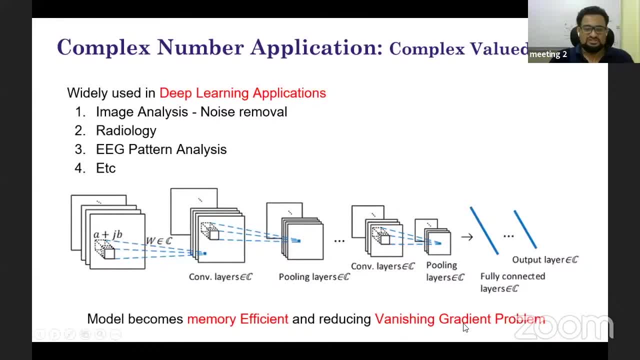 the vanishing gradient problem is a big problem which disturbs you in optimization. then the complex number gives you very good value. So that is one more very important thing- I was just forgetting it- to mention that the fraction module can reduce the vanishing means. it reduces your vanishing gradient problem. 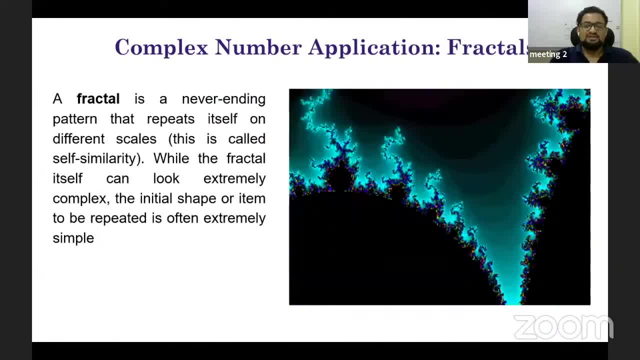 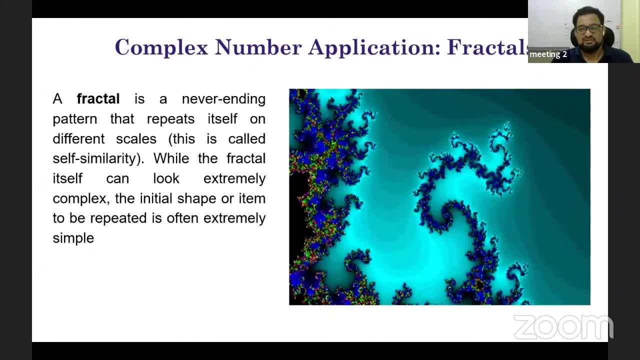 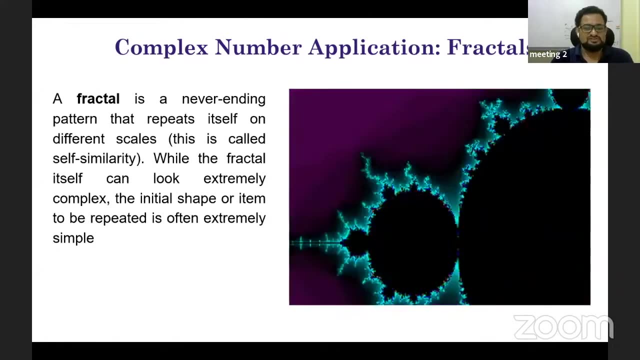 as well as it becomes, it makes your model more memory efficient. So another very important, a very wide application of this one complex number is used in the fractals. So a fractal. let me define a fact. I think yesterday you saw a few slides in Professor Nagbhushan Sir's. 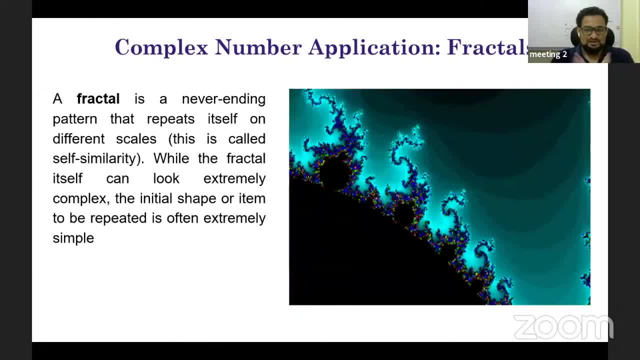 lecture. So let me, so now I tell you that see, yesterday you saw only picture, but today I am telling you that this lecture is way better than the last lecture. So let me, so now I tell you that see, yesterday you saw only picture, but today I am telling. 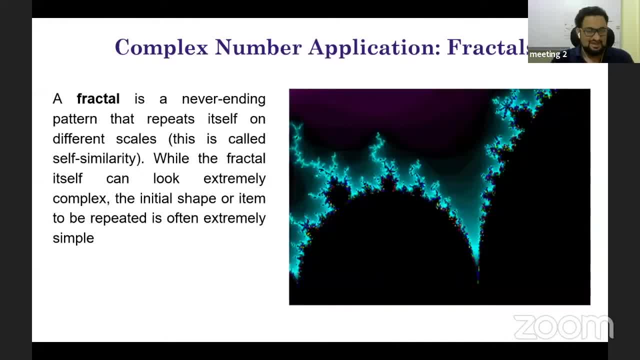 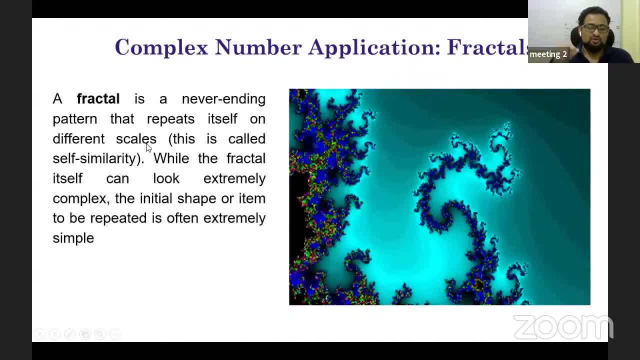 you that this can be used for a lot of applications, So we need to call it a problem, if you are interested. picture is derived from complex numbers, So a fractal is a never ending pattern that repeats itself on different scales. So when you see this, fractals are very popularly found in 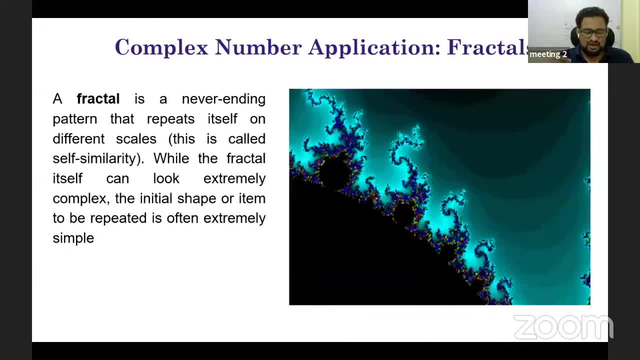 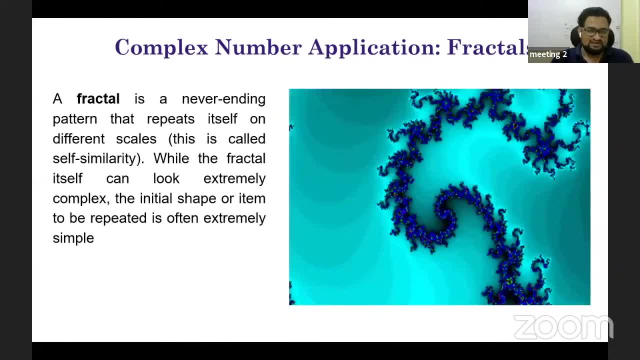 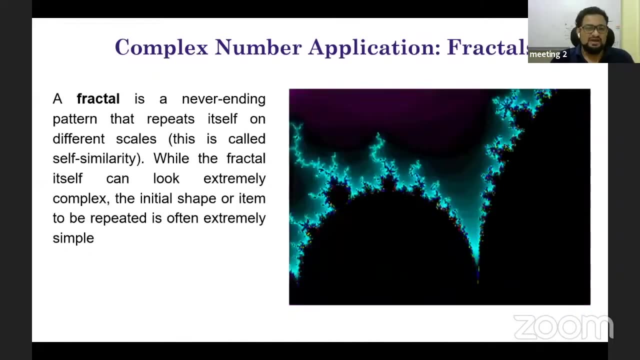 what you call, I think, in the snow, snowflakes, I don't know, I don't remember the exact word in snow, if you try to zoom. and so there is a separate book, textbook written on fractals. So if you go through that, the fractal is a never ending repeating pattern, that itself that it repeats. 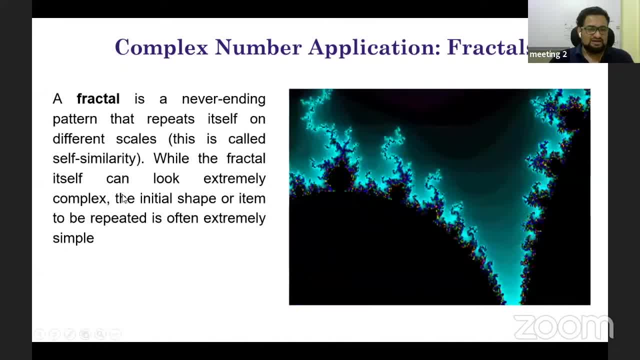 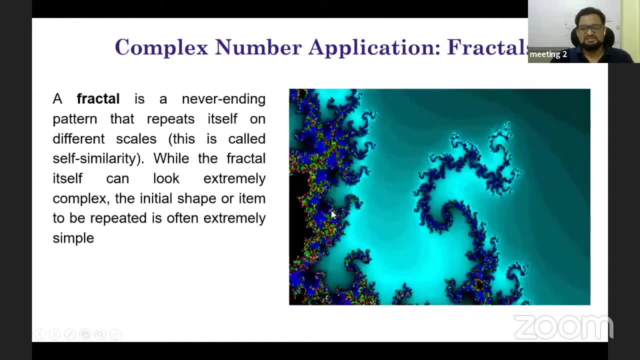 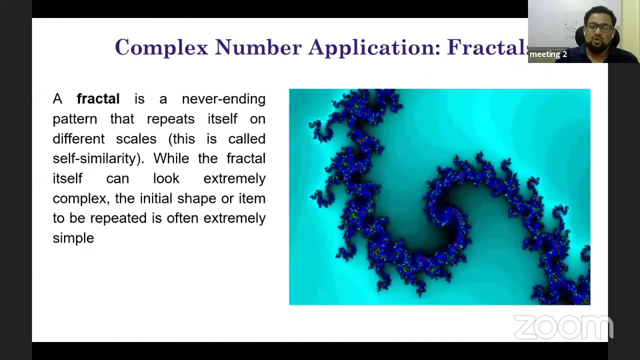 at different scales, same pattern. while the fractal itself can look extremely complex, the initial shape or the item to be repeated is often extremely simple. So this is the one basic example of complex numbers to represent fractals. Now you want to represent this fractal, so you need to use 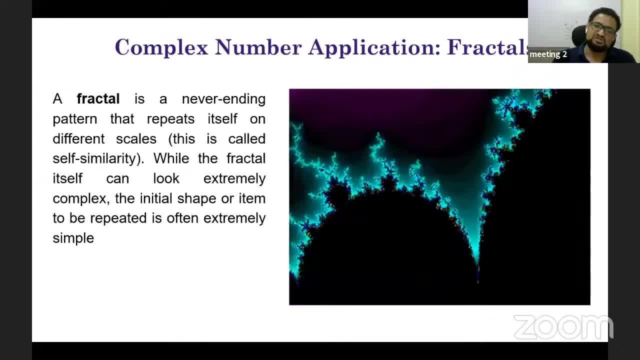 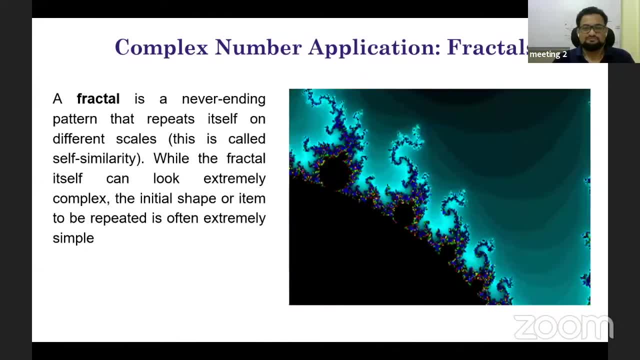 the complex numbers. So now you can generate these fractals by using visualizing the complex numbers. So two way: now you have a complex number you want to visualize, then you can generate fractals out of that. These are some of the. yesterday also you saw some slides related to this one: the objects in 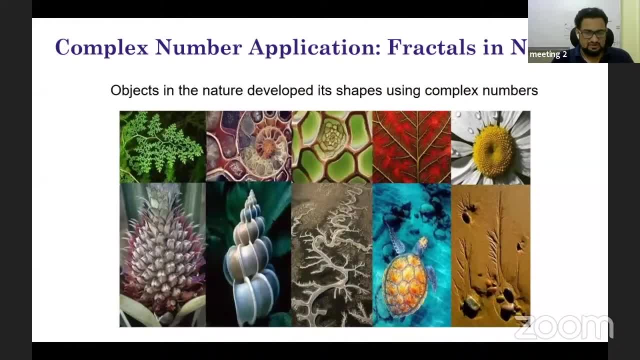 the nature develops is shape using complex numbers. Okay, so now this is the best example that your complex number has very wide application. the nature also thinks. that is why, like we have See, the main motivation is that in nature we find equations which require complex number to be. 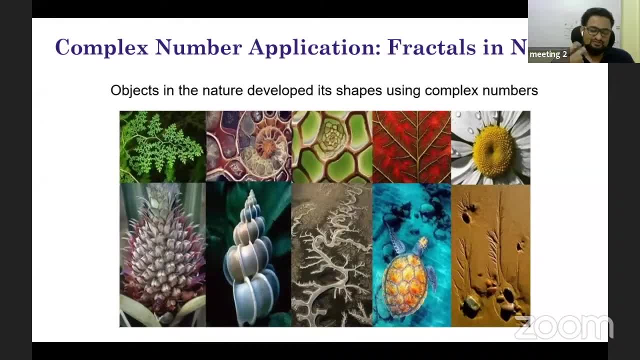 solved right. So, same way, the nature is also made up of different. okay, the nature is also made up of different objects which require the complex number representation. okay, the kind of objects which are shown here. Now, the complex numbers are also used in control theory. So I am. 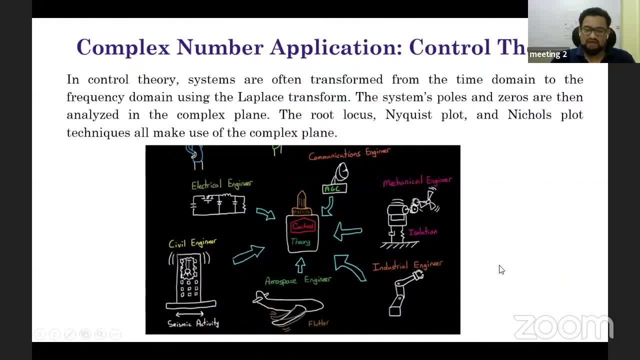 not an expert in the control theory, So I would. I would not go much into the details, but I can just tell you that in control theory everything like, for example, communication, means means all the objects, all the different entities need to be put together and bound together, and that is how the